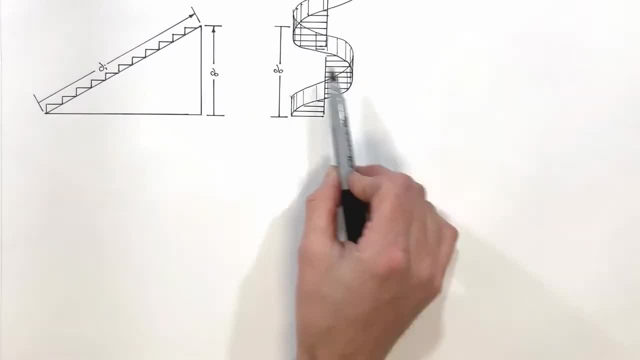 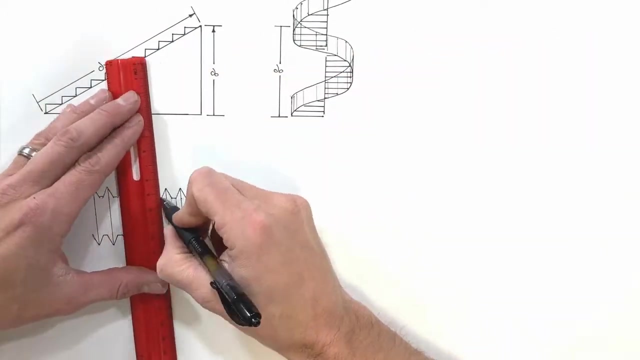 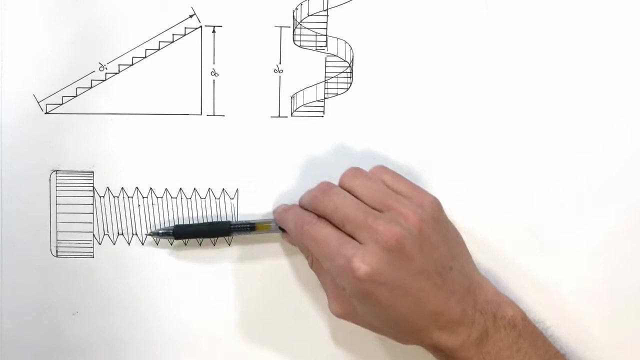 a screw is really nothing other than an inclined plane wrapped around a central axis, just like a spiral staircase. To get a better handle on screws, let's- let's take a look at a screw. So in looking at a screw, there's a screw or a bolt head, and then there's these threads, The threads. 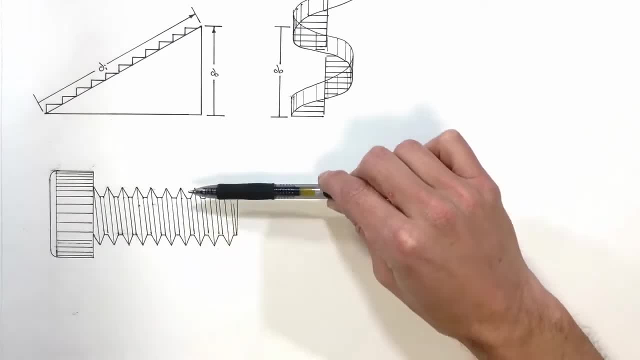 are really just a ramp that has been wrapped around a central axis, just like a spiral staircase. Now, rather than having little people try to walk up this screw, which I've turned on its side, what we do is we turn a screw and it is then driven into some base material like a nut or a. 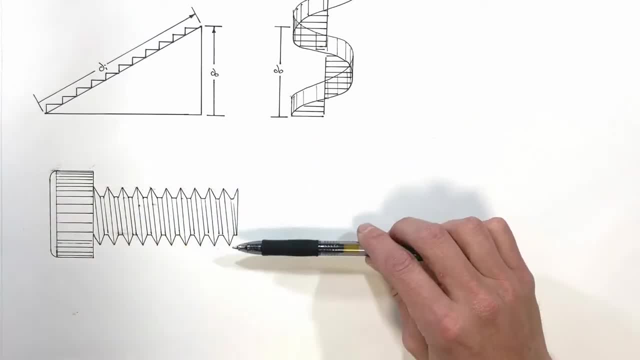 bolt or a cylinder head or whatever it is we're trying to to bolt into. So there's a few things we need to talk about with screws as far as vocabulary and nomenclature. To talk about with a screw is something called the pitch of the screw. 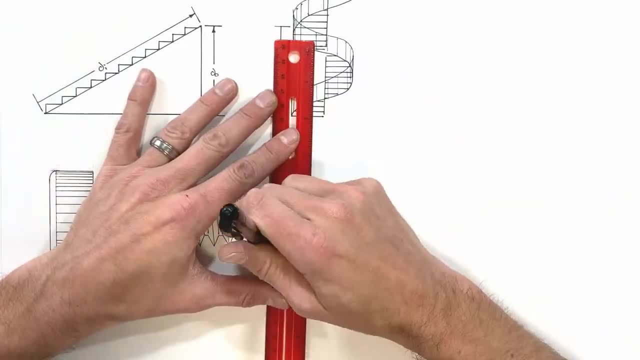 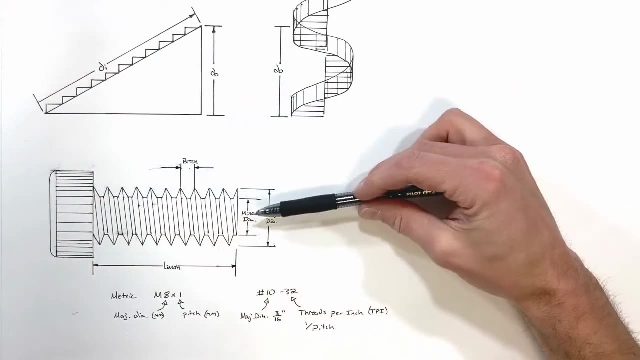 Okay, so we have a bolt and there's a couple different dimensions that we care about with this. There's the pitch and this is the distance from one thread to another. Or, if you go back to our spiral staircase, this is really the distance traveled vertically on our spiral staircase. 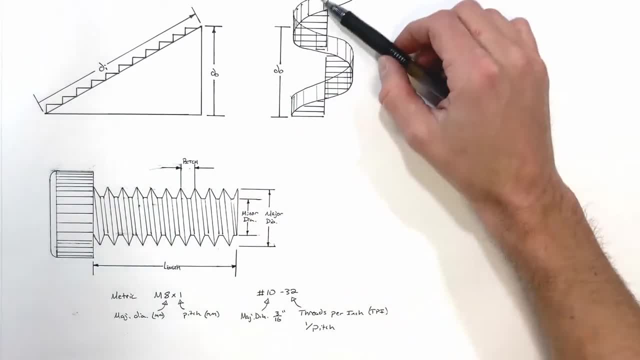 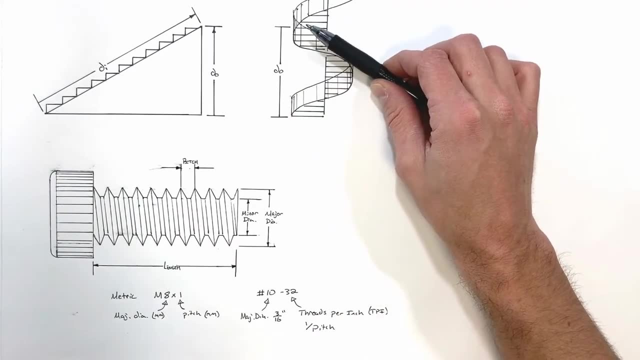 if we were to walk around it once, Going back to a screw, if we were to turn the screw, it would be a little bit more difficult to get the screw to go up and down. So if we were to turn the screw, it would be a little bit more difficult to get the screw to go up and down If we were to turn the screw. 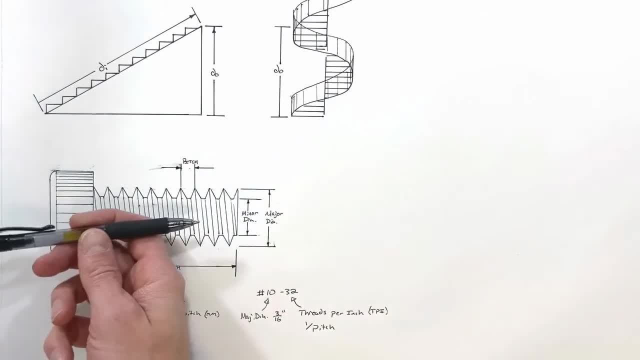 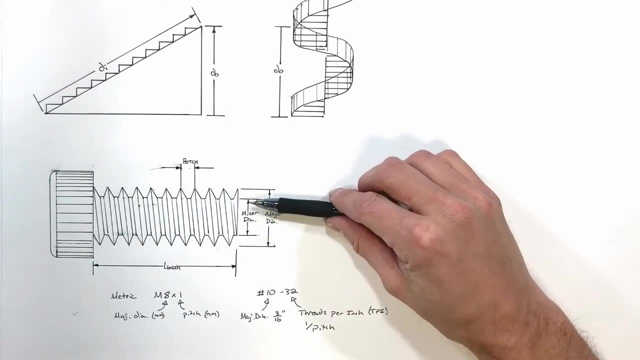 or bolt around. one time it would move into a base material a distance equal to one pitch. Now we've got some other dimensions here. there's something called the minor diameter and the major diameters. These don't really play into how a bolt is used as a simple machine, but these are just 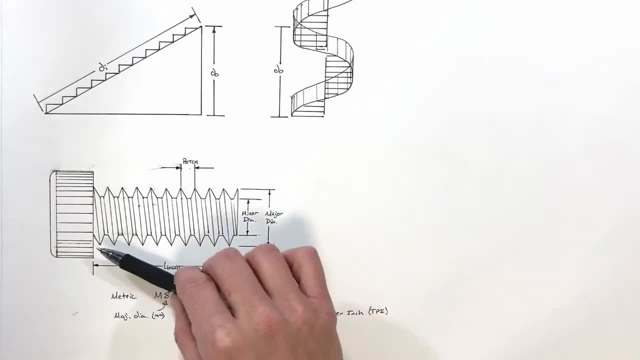 different ways to differentiate one bolt or screw from another. Then, of course, we have the length, and that really is just telling us how far into some base material this, this bolt, can extend. Now there are a couple of things that we want to talk about with this. First of all, we want to talk about 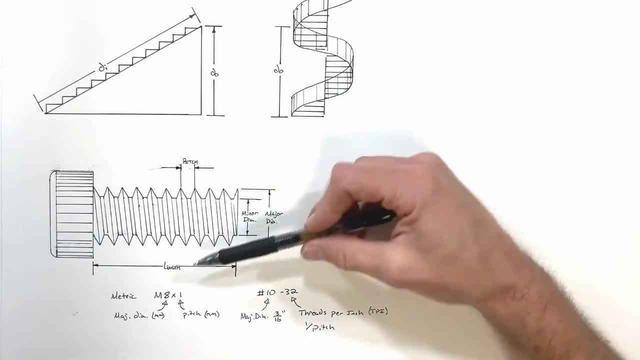 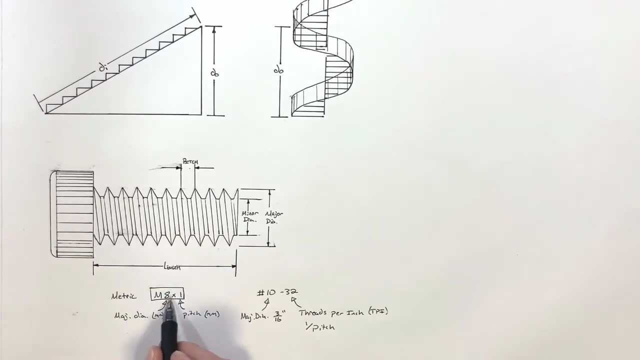 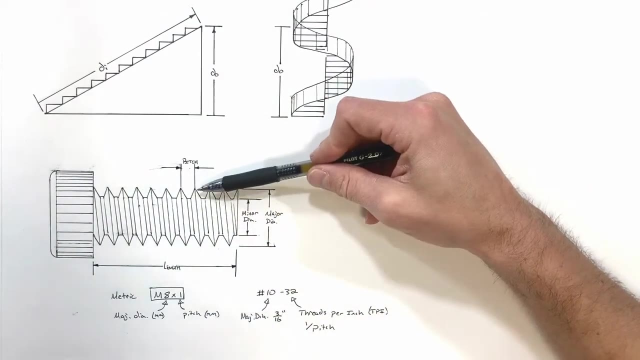 different types of bolts. We have metric bolts and then we have standard bolts. Metric bolts: they're pretty easy to deal with. When you look at a metric bolt, you'll see something like this: m8 by 1, and what this is telling us is the major diameter and the pitch, The pitch being how far. 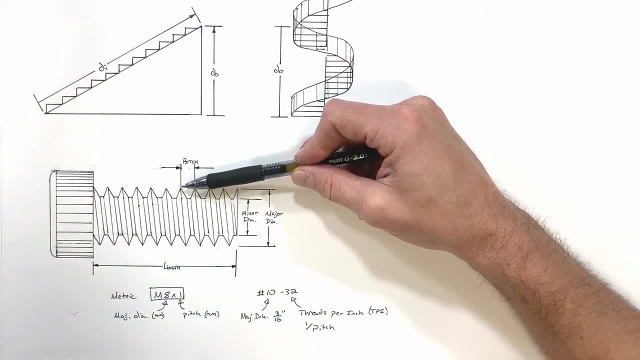 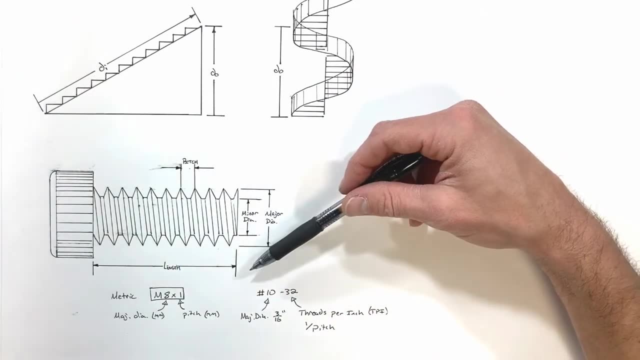 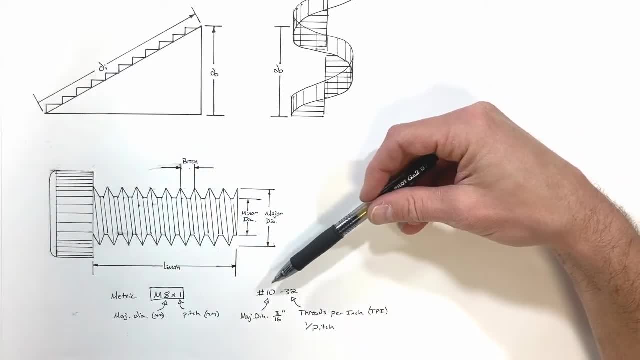 Then we have American units, which are a little bit more of a pain, because if you look at a bolt, go down to your, your local hardware store. what you'll find is something like a number 10-32 bolt or screw, and what this is is telling us about the major diameter, but it doesn't use. 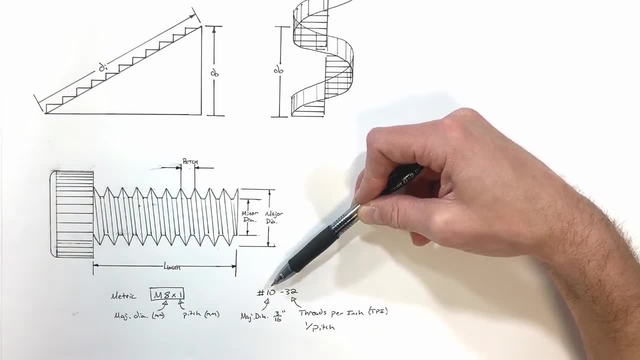 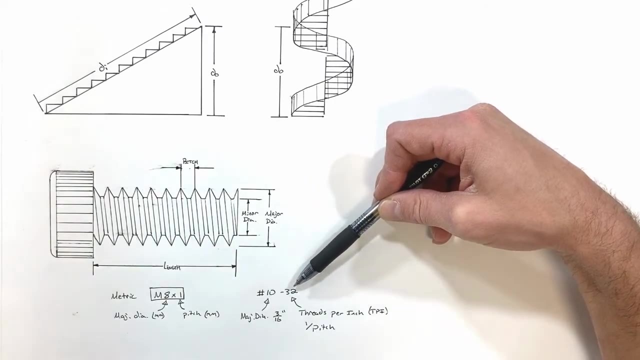 actual dimensions. it just uses a scale, kind of like gauges almost, and this is a major diameter of 3, 16 for a number 10 bolt. If you were to have a number 8 bolt, that'd be something a little bit smaller for the major diameter. Then this 32 right here, this, this isn't pitch 32 as a pitch would. 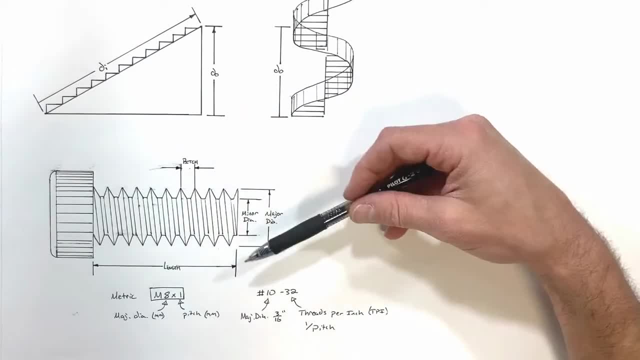 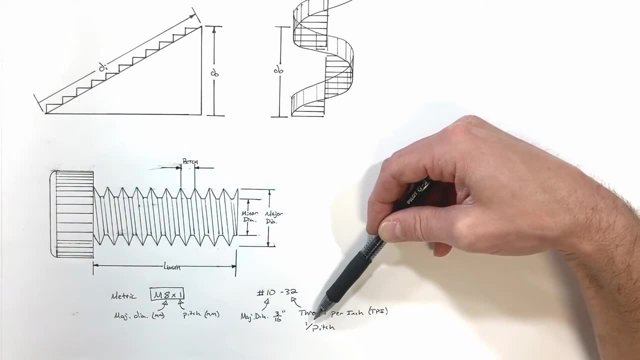 be ridiculous. that would be something like one thread every 32 inches, which would be functionally worthless. What this is is the threads per inch or tpi, and all that really means is this is one over the pitch or it's the inverse of the pitch, but again, when we keep you. 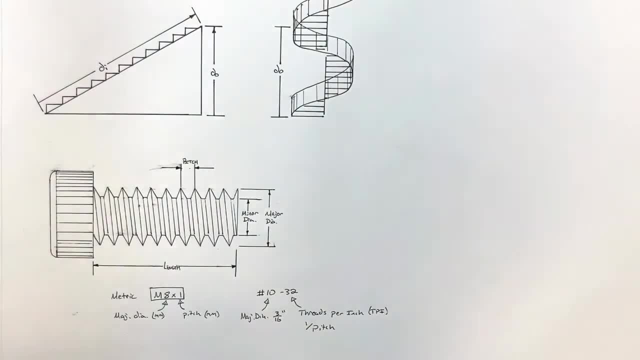 know American units, they're American units. it just keeps you confused. What can I say? So let's actually take a look at a bolt as a simple machine here. Okay, what I want to do in this problem is is take a wrench and put it on a bolt and run this bolt. 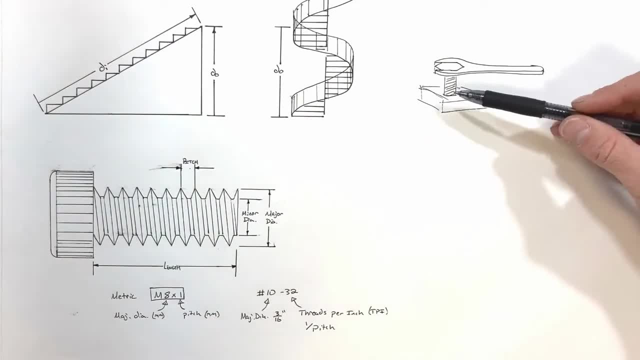 into some base material. This could be whatever it is you want. this is a screw going into a door frame or a bolt holding on some little piece of your bicycle? I don't know. I'll let you choose this scenario here, but what I want to do is look at this bolt with the wrench together as a simple 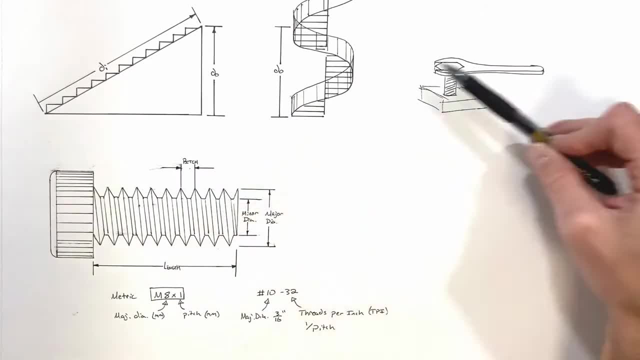 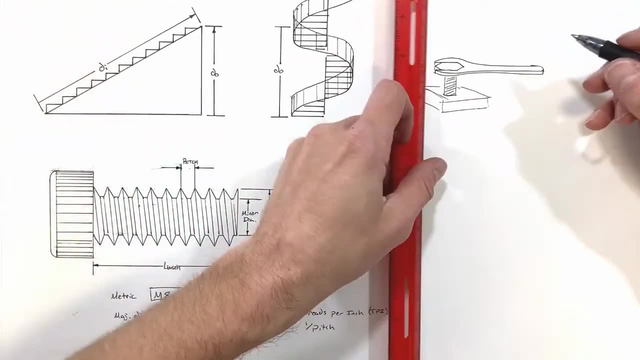 machine, because really a bolt on its own is not a simple machine. we have to turn it and we use a wrench to do that, so the dimensions of this wrench will actually come into play. So what we're going to do here is look at this wrench as having some length. 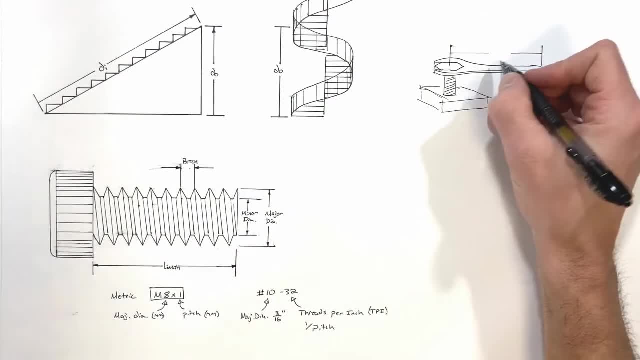 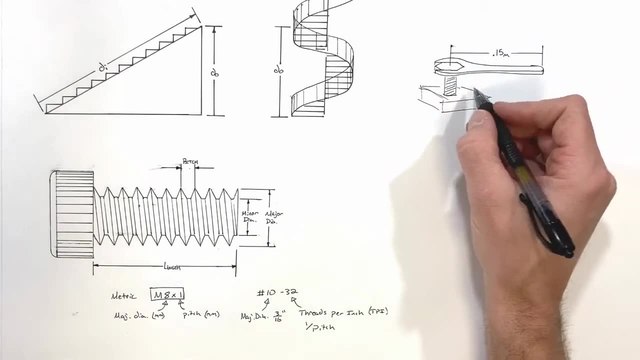 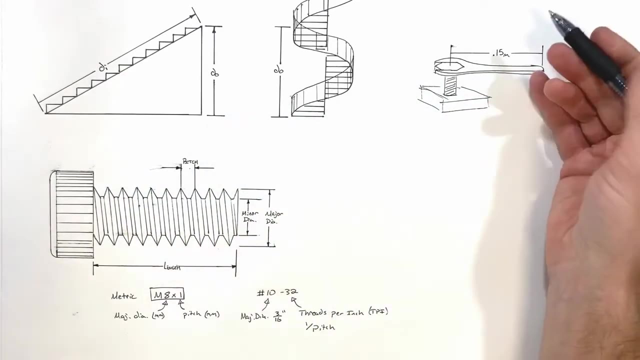 and because American units are silly, let's go through and let's just look at this in metric units. let's say this is a 0.15 meter long wrench, it's about six inches- and let's say the pitch of this bolt or the thread pitch, kind of like what we see over here, let's make this one millimeter, that is 0.001. 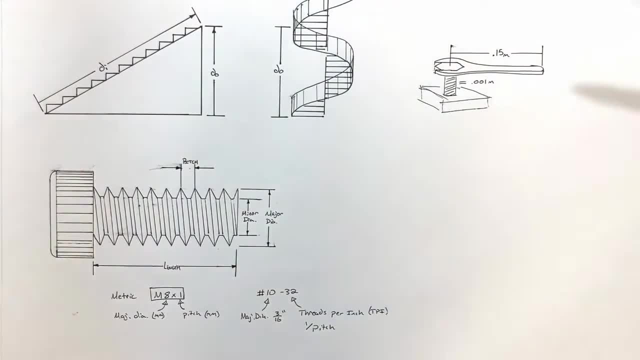 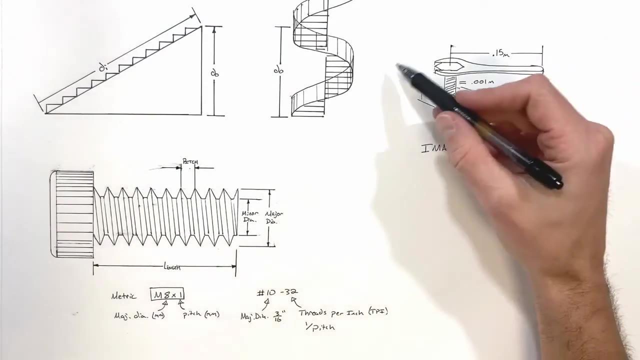 meters. okay, so what we're going to solve for in this problem, then, is the ima, or the ideal mechanical advantage of the system. now, you remember, ima is d in, over, d out, and ultimately what's happening is we're turning this wrench, so we're going to have to move this. 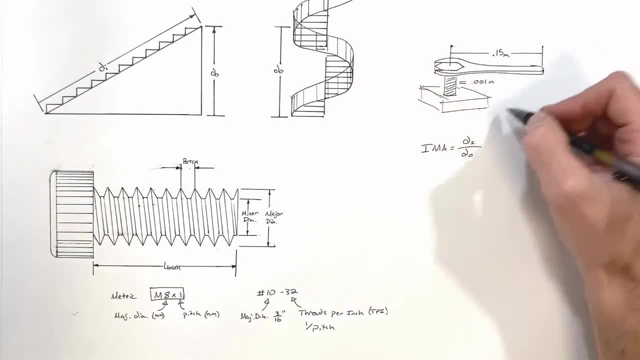 thing in a long ways. this wrench is going to move a long ways in a circle due to some force we're going to apply to it. so we're going to put some force tangent to this wrench that's going to cause it to move in a circle. as a result, this bolt is going to move downward into the space material. 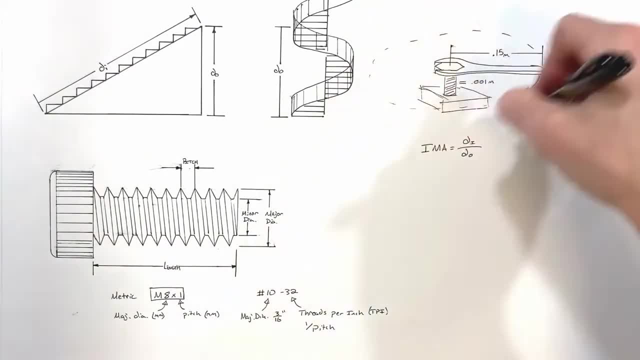 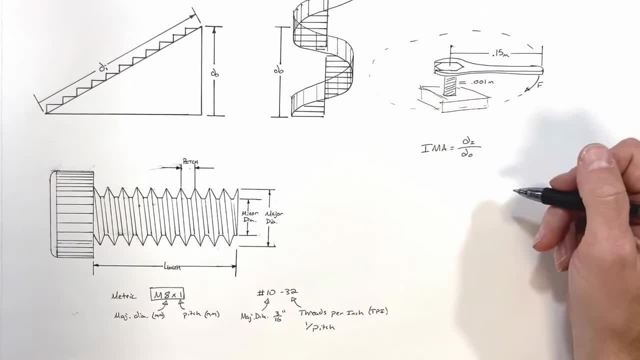 realize. let's just look at turning this wrench around one single time, and we know, if we turn this wrench around one single time, the end of the wrench, or where we're applying this force, is going to travel one circumference around this circle, and we know circumference is 2 pi r so 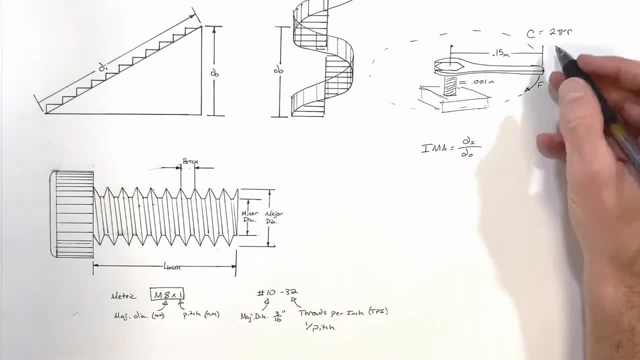 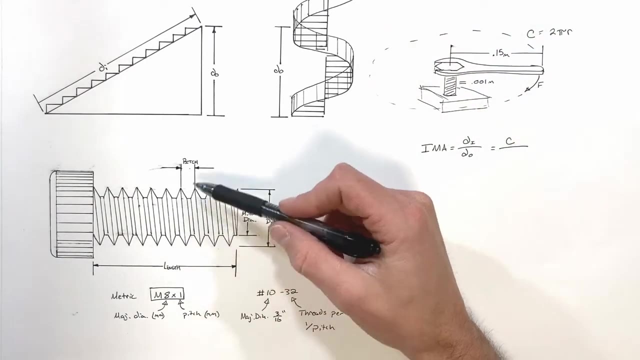 let's treat the input distance from one single revolution as just being 2 pi r, so that means we're the circumference, that's the input distance. now the distance which this bolt travels into the base material, going back over here is going to be the pitch. remember a bolt will travel into a base. 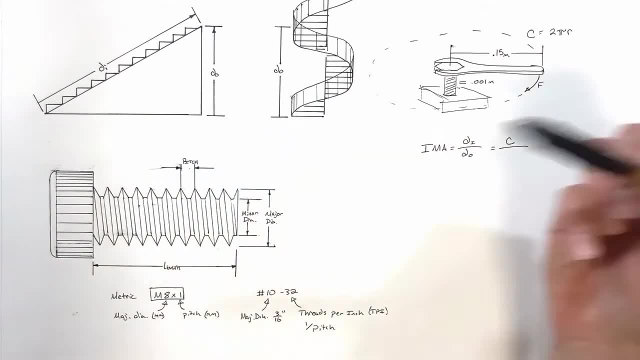 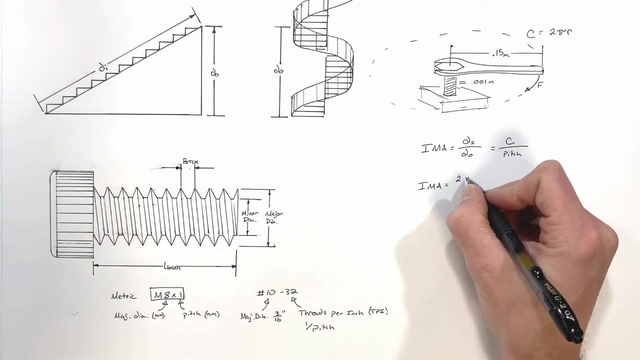 material, one pitch in length for every revolution. so the circumference over the pitch is simply going to be the ima of this simple machine. so the ideal mechanical advantage of a bolt in this case is going to be 2 times pi, times 0.15 over the pitch of 0.001. now this works out to be 940.. 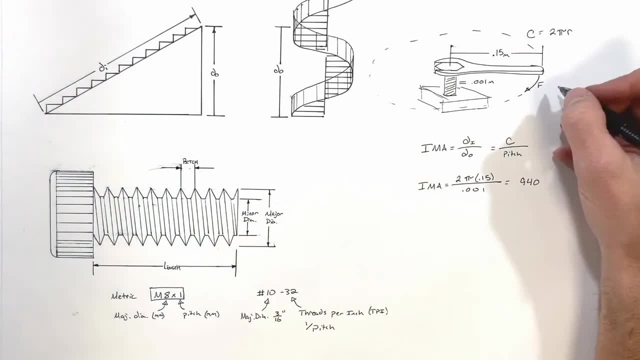 that's an enormous ima. what this means is, if we were to put a force on this of 10 newtons, i realize that's roughly two and a half pounds. looking at this, this ama now, assuming this was 100 percent efficient, the ama being f out over f in. 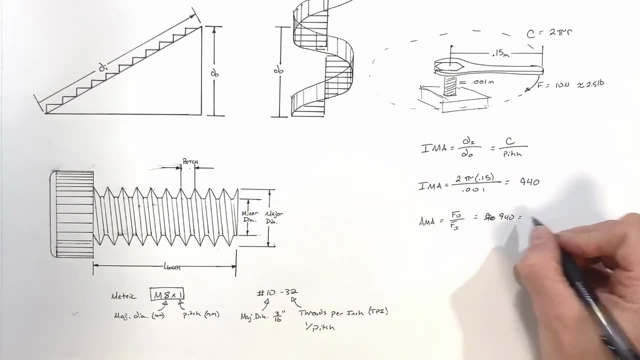 if this was 100 efficient, we would have an output force over 2.5. in this case, the output force works out to be an enormous 23, 50 pounds. so by pushing with just two and a half pounds of force on the end of this wrench, 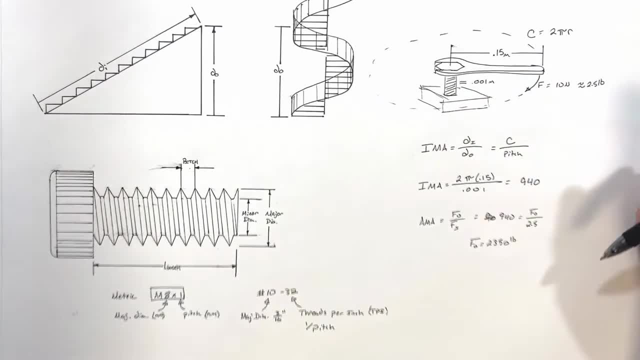 we're able to create a huge clamping force between this bolt and this base material, now in reality a screw and a bolt. it's not 100 efficient, so we might only get a fraction of this, but even still, putting in just a few pounds to get hundreds or thousands of pounds of. 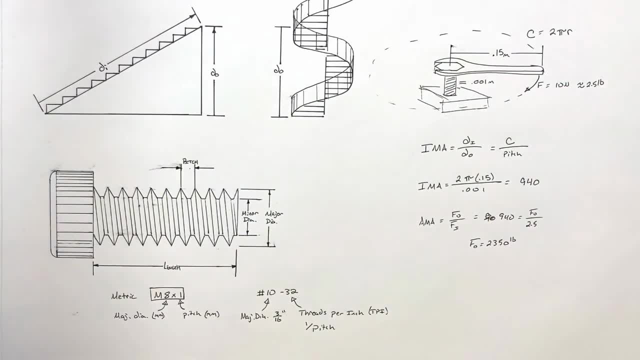 clamping force out of this makes this an extremely useful, simple machine. so, in summation, we should see that a screw or a bolt is really nothing other than an inclined plane. it's important that we understand the vocabulary, especially understand what a pitch is for a screw. 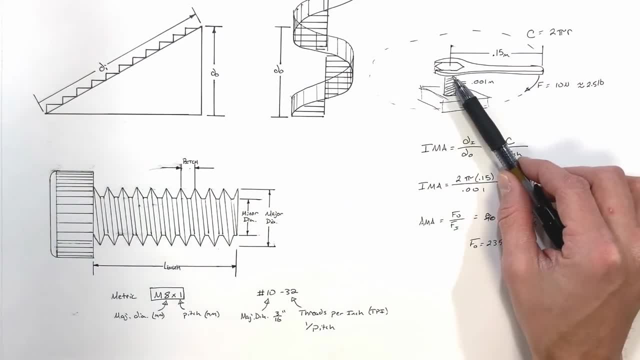 or a bolt. and i want you to realize, when looking at a screw or a bolt as a simple machine, we really need to take into account a wrench or a lever that's acting on the screw machine. the ima for a screw or a bolt it's always going to be really high, it's really large. 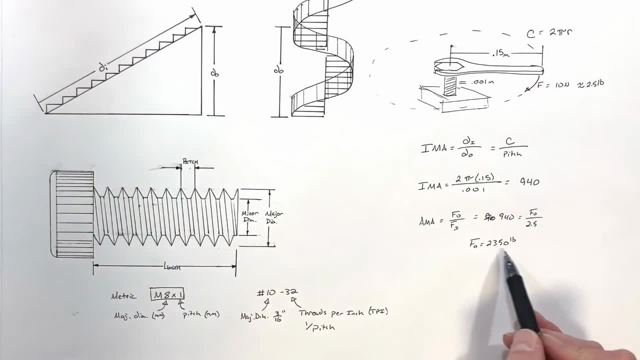 this is why we use screws and bolts. in reality, the ima is never going to be the same as the ama, and that's because the screw and a bolt isn't particularly efficient. there's quite a bit of friction between these threads and a base material, but still we get. 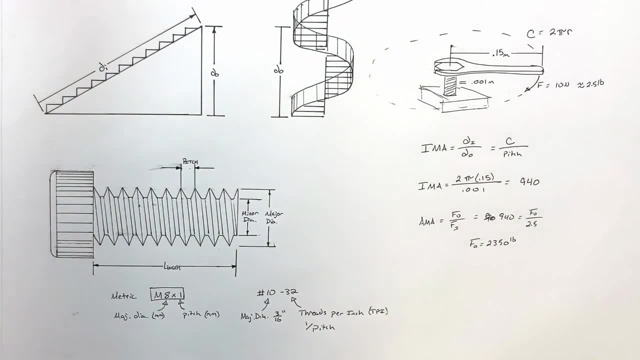 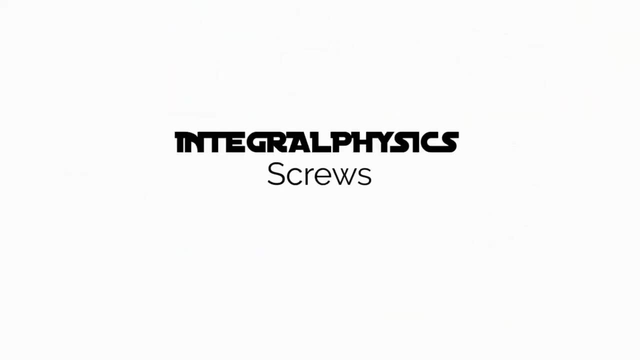 enormous forces for relatively small input forces. and, on that note, that's all for now.